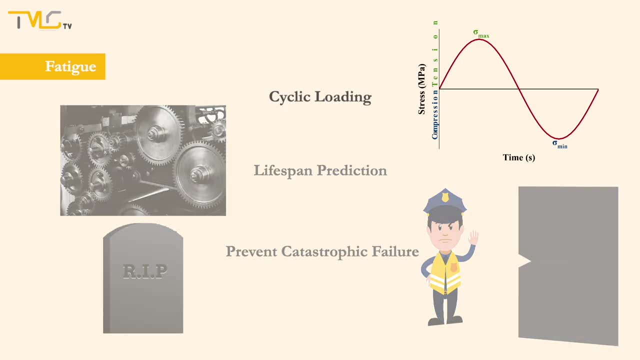 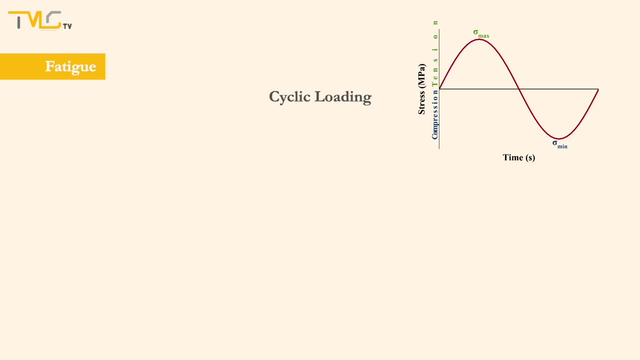 failures. Briefly speaking, fatigue can be defined as a type of failure that occurs in structures subjected to cyclic loading. For most of the metals, including ferrous and non-ferrous alloys, fatigue is the most commonly observed reason for failure. In addition to that, 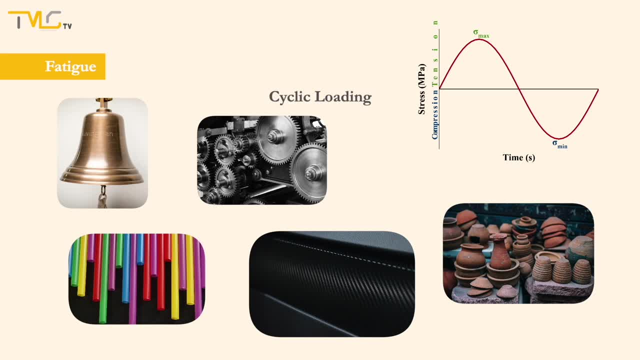 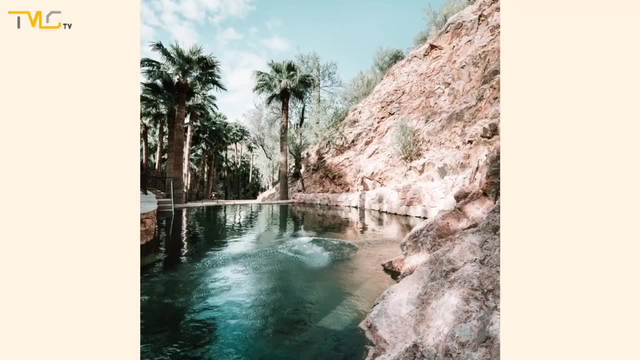 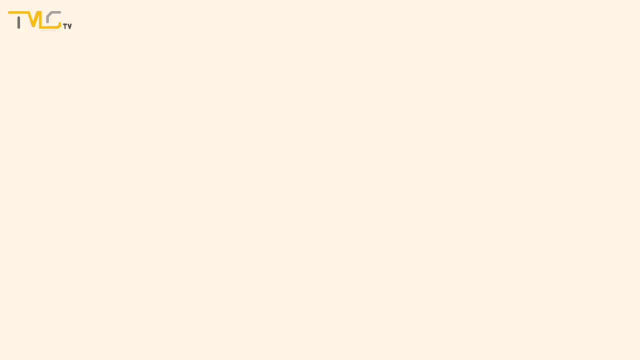 ceramics, polymers and composites can experience fatigue failure as well. Before diving into the depths of fatigue concepts, let's initially get more familiar with fatigue failure. There are three important factors causing fatigue failure, which are high tensile stresses, large variation in the applied stresses and a great number of cycles of applied stress. 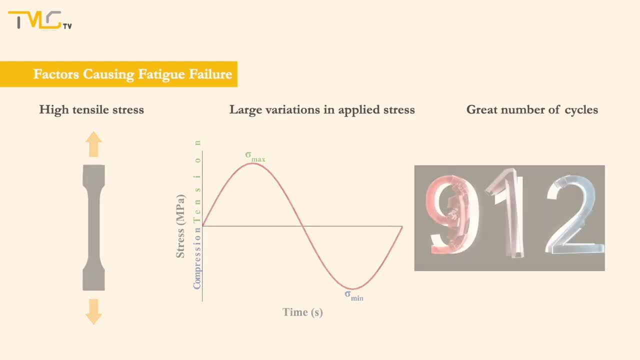 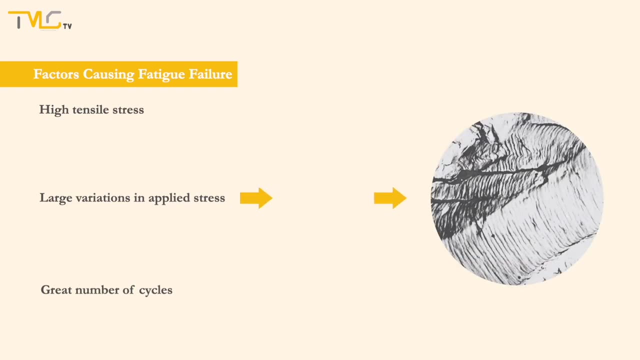 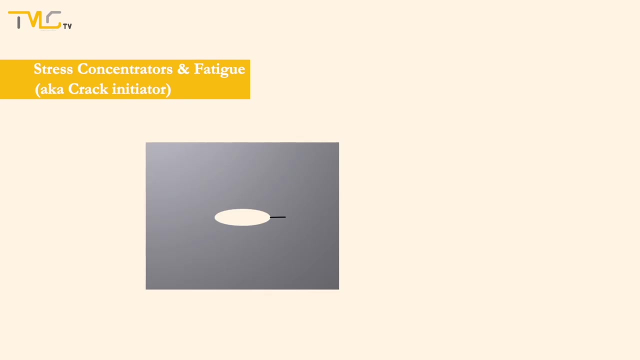 So how do these factors lead to fatigue failure of a material? Fatigue fracture occurs at three main steps, namely crack initiation, crack propagation and final sudden fracture. Fatigue cracks always initiate at stress concentration points, also called as crack initiators. Local stresses at crack initiation sites are considerably higher. 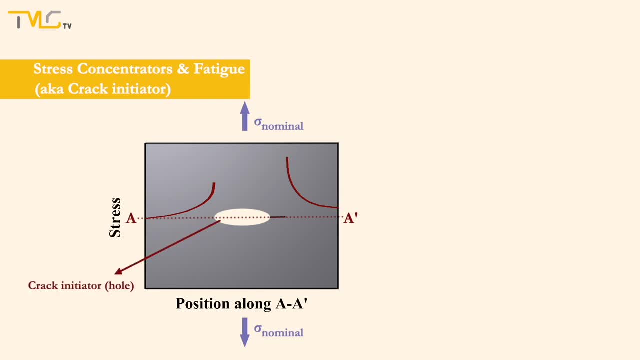 than nominal stress. You may recall the crack stress amplification relation from video number 2.2.. A wide variety of surface heterogeneities can act as stress concentrators. Such heterogeneities are significantly important for the detection of potential stress concentration points and for monitoring the crack initiation and later. 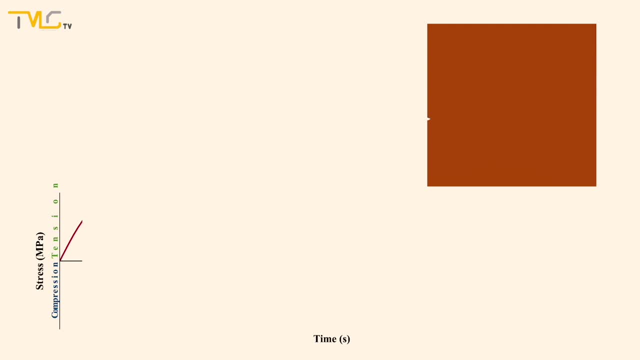 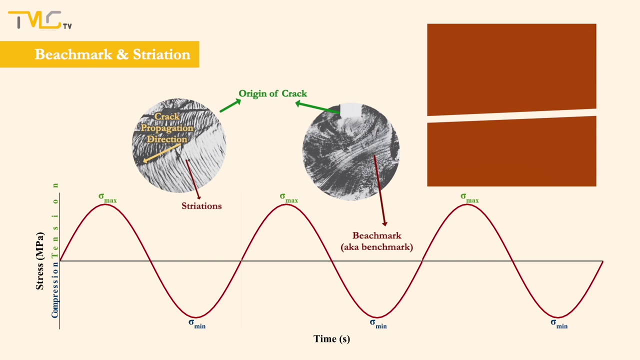 propagation. Once formed, cracks progressively advance and grow under cyclic loading. Two types of markings can be seen at the fracture surfaces of the fatigue-filled material, namely beach mark patterns and striations. Both these markings are seen as concentric ridges advancing from the origin of the crack. 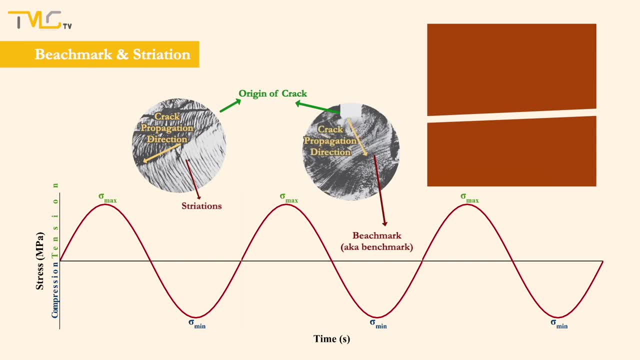 through the cross section of the material until fracture Beach-mark patterns are beg vom Estático, where asin it is as same as transverse bezel tiles. Above that, the fear, the drop-in and the angry scared 175° movement are Lauqu¿ início the proper". 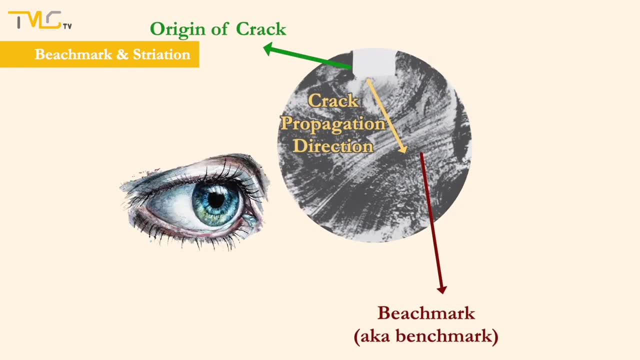 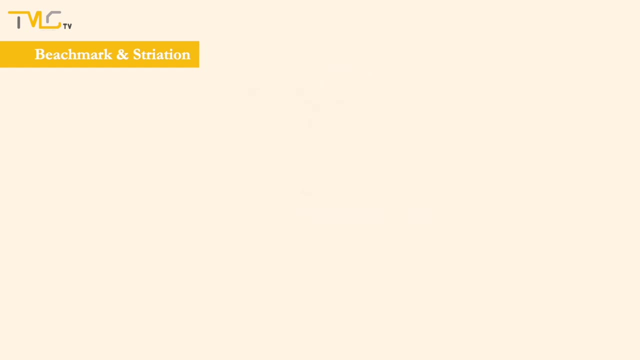 Beachmark patterns are macroscopic markings and they can be seen by naked eye without the aid of any optical equipment. Each beachmark pattern indicates a period of time over which crack growth occurred. Fatigue striations, on the other hand, are microscopic and can be observed under electron microscopes. 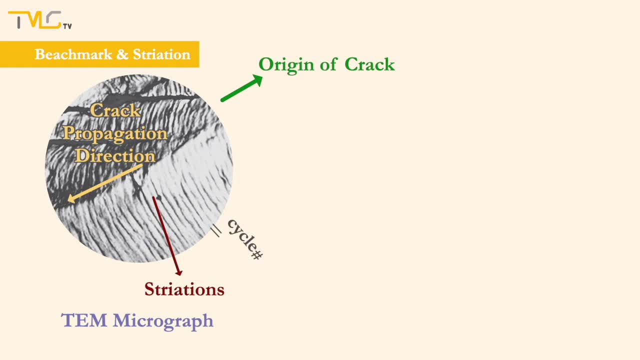 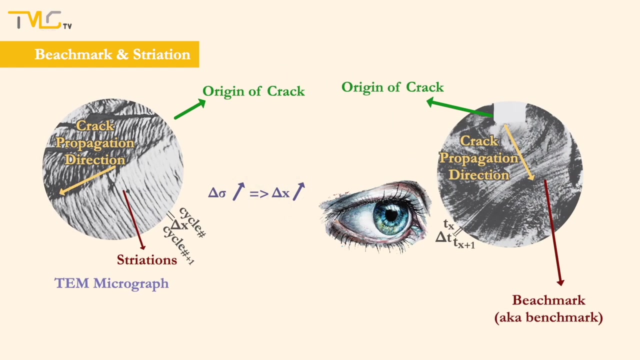 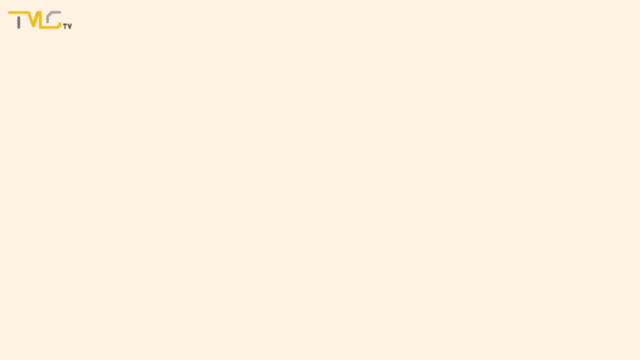 Each striation mark represents the propagation distance of a crack during a single loading cycle. Striation width increases with increasing stress range. Although beachmark patterns and striations look alike, they differentiate in terms of size and origin, with different fracture characteristics. After explaining the reasons and fracture mechanisms of fatigue phenomena, we can now focus on the driving force of fatigue. 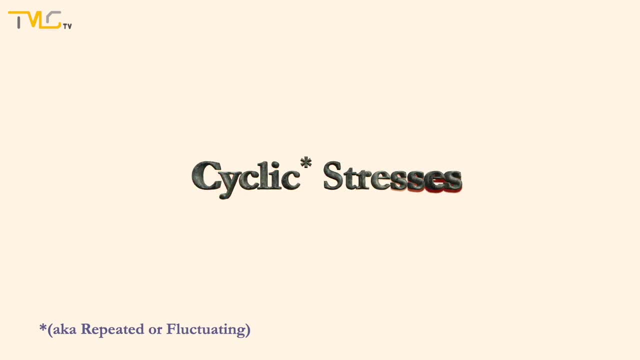 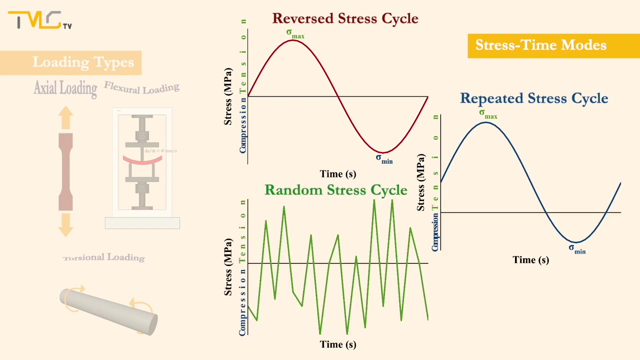 You may also know them by the name of cyclic stresses. Components under service can experience three types of loading: axial, flexural and torsional- And these loading types produce three different cyclic stress time modes: reversed stress cycle, repeated stress cycle and random stress cycle. 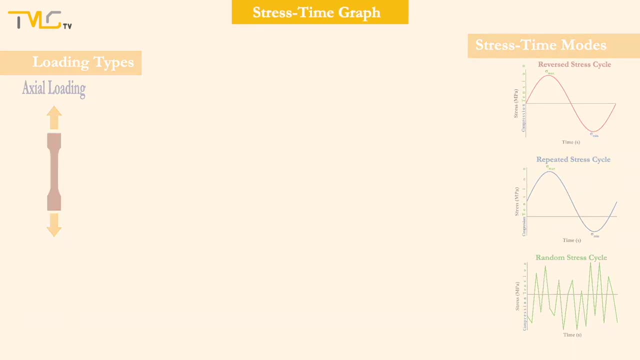 Since the beginning of this video, you kept repeatedly hearing the phrase cyclic loading. But what is that? Now let's take a look at the stress-time curve of a specimen tested under fatigue loading conditions. On the y-axis of this curve is the applied stress in MPa, shown as positive for tensile and negative for compressive loading. 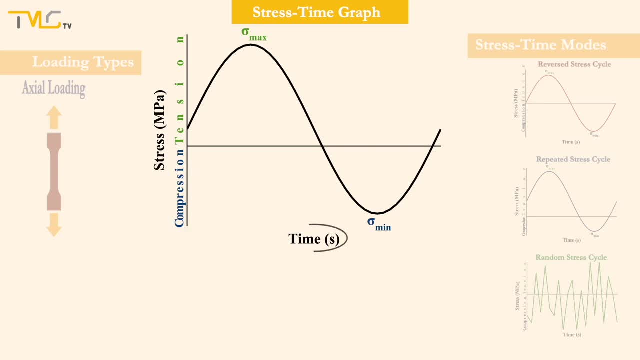 And on the x-axis is time showing the duration of the exposure of MPa and the material to the varying stress values under cyclic loading conditions. The maximum stress shown on the stress-time graph is denoted as sigma max and minimum as sigma min. 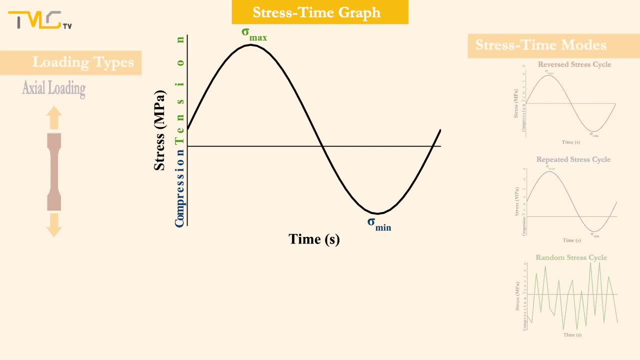 and both are reported in MPa. Using these max and min stress values, mean stress, range of stress, stress amplitude and stress ratio can be determined easily. Mean stress is denoted as sigma m and is reported in MPa. and is equal to the average of maximum and minimum stresses in the cycle. The range of stress is denoted as sigma r and is reported in MPa, and simply stands for the difference between sigma max and sigma min. Stress amplitude is denoted as: 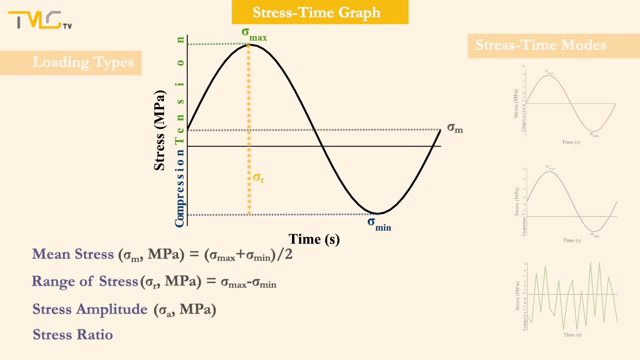 sigma a and reported in MPa, and defines the amplitude of the applied maximum and minimum stress values with respect to the mean stress and is equal to the half of the range of stress value. Lastly, the stress ratio is denoted as: 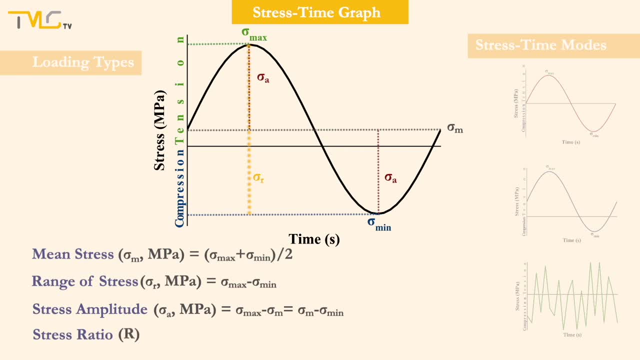 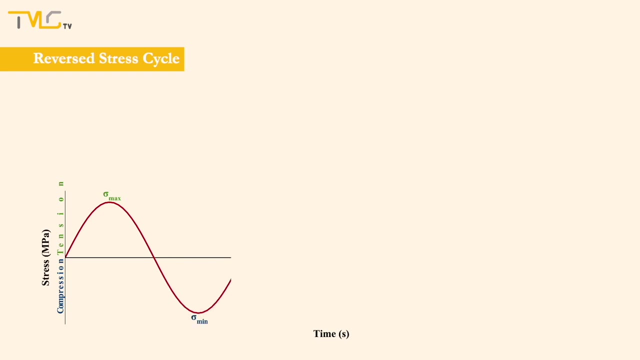 r and is the ratio of minimum stress amplitude to that of the maximum stress. Now let's move on to the cyclic stress-time modes. Reversed stress cycles show regular and sinusoidal time dependence and are reported in MPa, and both are reported in MPa. 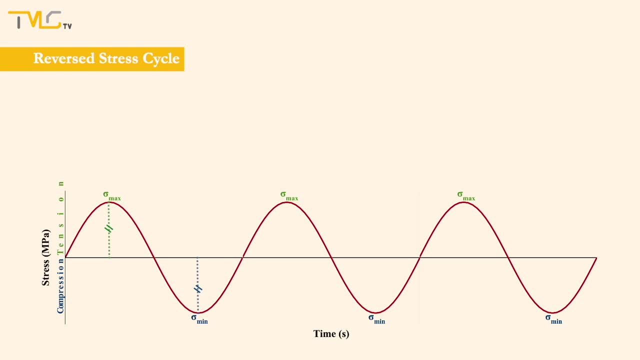 The stress ratio is denoted as sigma r and is reported in MPa, and is the ratio of minimum stress amplitude to that of the maximum stress value. In other words, stress alternates from a maximum stress in the tensile region. 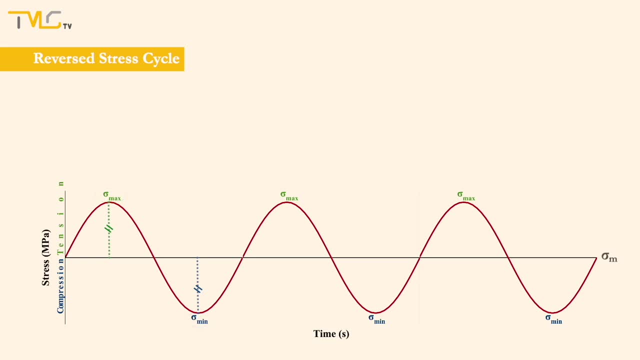 to a minimum stress in the compressive region. Both of these stresses have the same stress magnitude, but they are acting in the opposite directions. Therefore, in reversed stress cycles, mean stress is equal to 0 MPa and the stress ratio is equal to. 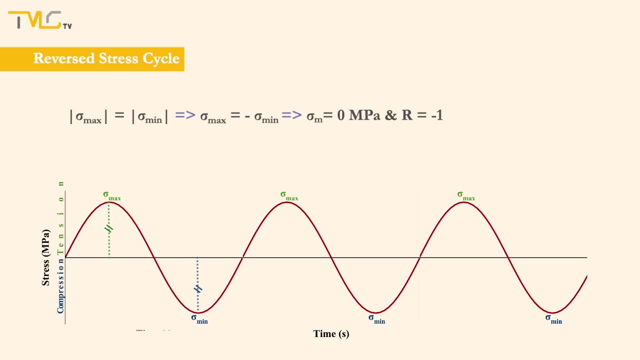 minus 1 MPa. One fatigue cycle is composed of tensile loading, tensile unloading, compressive loading and compressive unloading for a reversed stress cycle. In repeated stress cycles, the maxima and the minima are asymmetrical relative to the zero stress level. 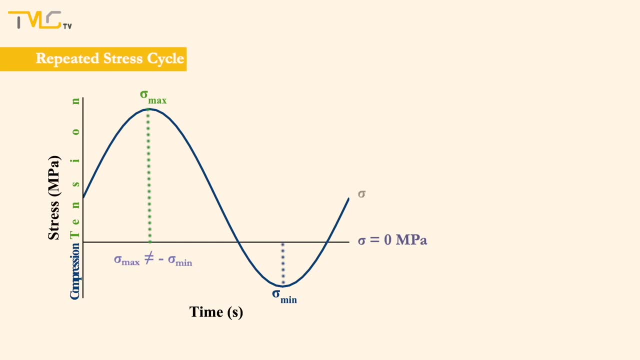 as shown in the image on the screen. Here, the mean stress and the stress ratio are equal to any value other than 0 MPa and minus 1 respectively. The last stress time mode observed in fatigue loading is the random stress cycle. 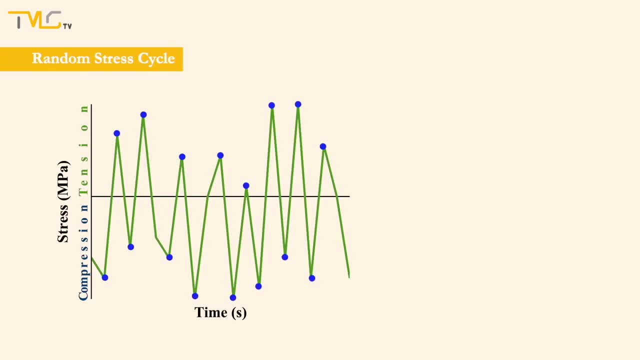 in which the stress level may vary randomly in amplitude and frequency. Hence we cannot talk about a constant mean stress range of stress, stress amplitude or stress ratio values Similar to the applied stress amplitude and frequencies. they will fluctuate too. 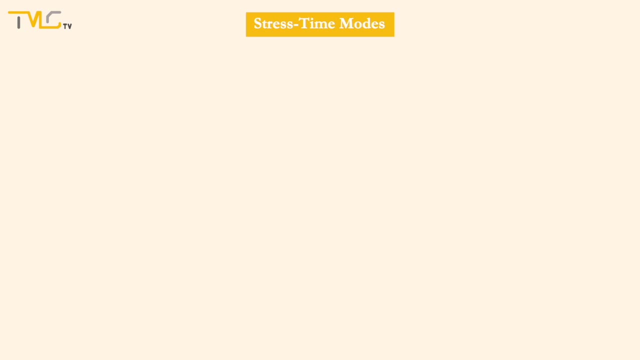 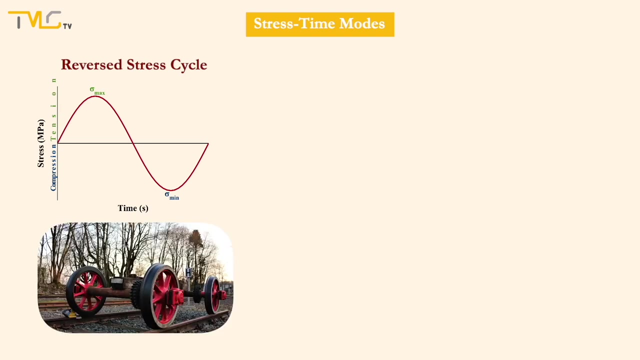 Before finishing this video, one example for each stress time mode will be given. The rotating shaft of a train to which bending loads are applied in a cyclic fashion experiences a reversed cycle fatigue during operation. A loaded spring is already experiencing tension and the magnitude of tensile stress may decrease.